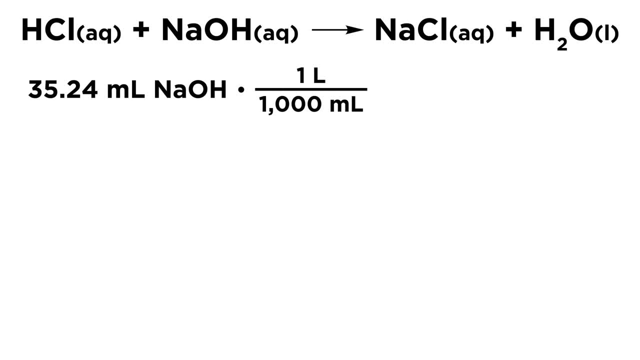 required to reach the equivalence point. and let's first convert that into liters. So, dividing by a thousand milliliters, we have 0.03524 liters of base to reach the equivalence point. Now, since we have the concentration of that base, we can. 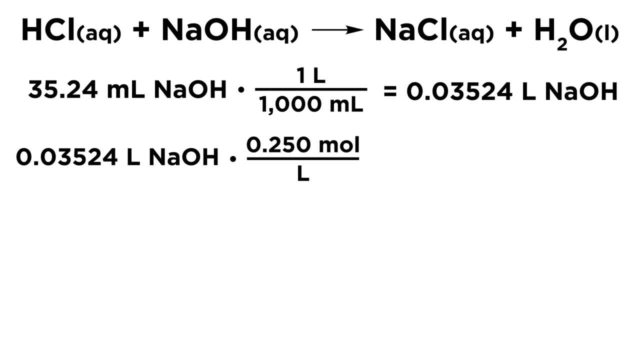 convert liters into moles. So let's take our liters of base and multiply by 0.250 moles per liter, And that means that was 0.00881 moles of base that were required to reach the equivalence point. Now we have to look at the stoichiometric ratio. The acid and the base are in a 1 to 1 ratio. 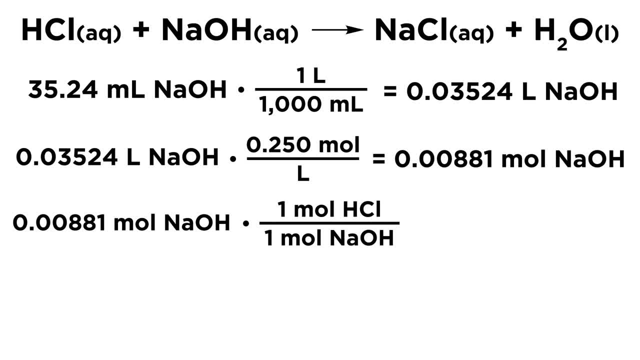 So that means, if that many moles of base were required to reach the equivalence point, then we multiply by 1 mole of acid over 1 mole of base and we get that same number of moles back for the acid. So when the equivalence point was reached, that many moles of base. 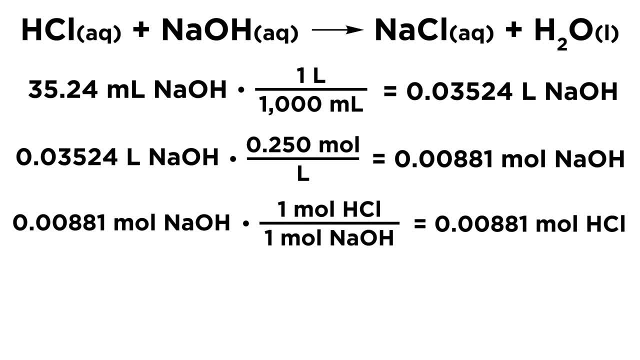 had precisely neutralized that many moles of acid, And that is the number of moles of acid that were in the solution initially for the HCl solution. So now all we have to do is convert that many moles of acid into a concentration, and so 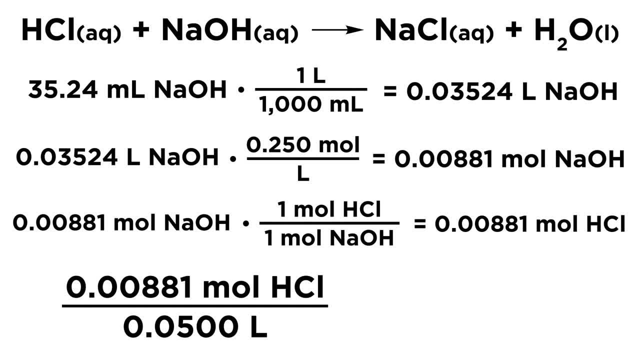 we can see that the concentration is moles per liter. So we take our moles of acid and we divide by 0.0500 liters, because we know we had 50.0 milliliters of acid. We knew the volume, we just didn't know the concentration. So that many moles over that many liters gives. 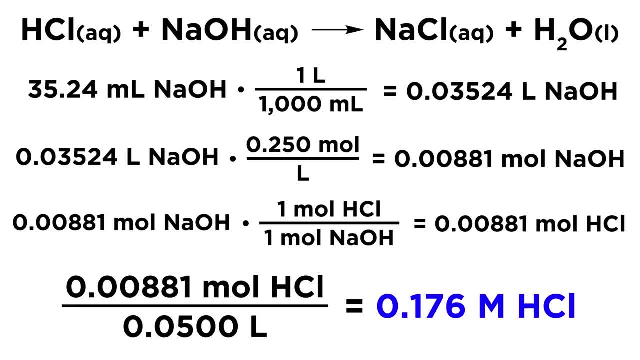 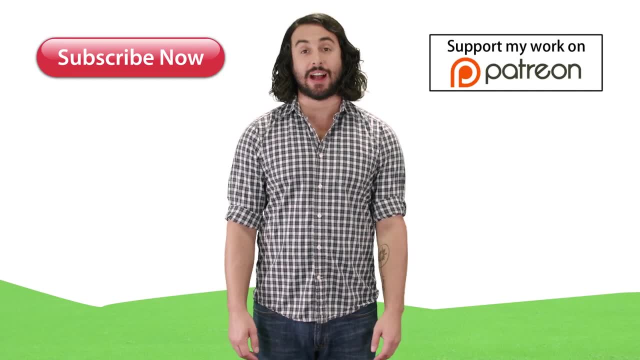 us 0.176 moles per liter, or 0.176 molar HCl, which was the concentration of our unknown HCl solution. Thanks for watching, guys. Subscribe to my channel for more tutorials. support me on patreon so I can keep making. 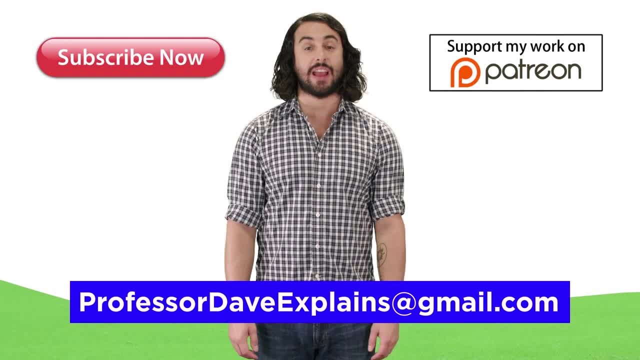 content and, as always, feel free to email me professordaveexplains at gmailcom.